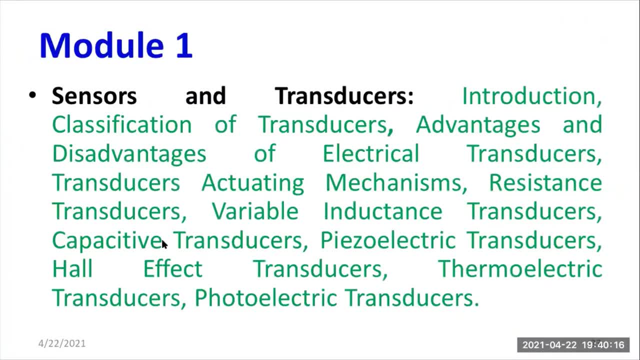 be discussing in the forthcoming days. First, in the foremost, I'll be discussing about: what do you mean by sensors? What is the difference between sensors and transducers? How do you classify the transducers? Then the pros and cons of electrical transducers, Then transducer. 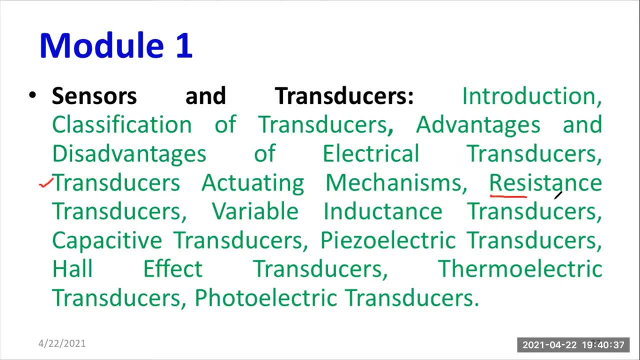 actuating mechanism, Then different type of transducers, such as resistance transducers, variable inductance transducers, capacitive transducers, piezoelectric transducers, Hall effect transducers, thermoelectric transducers and, finally, four-way transducers. 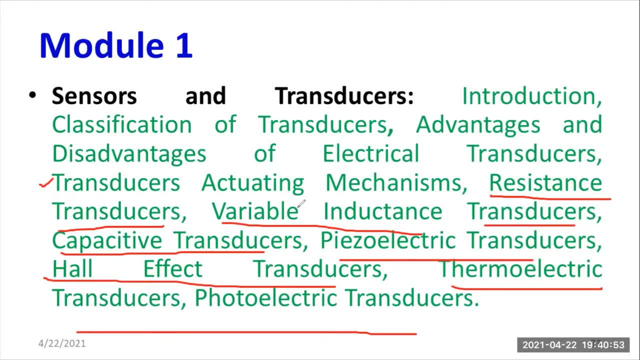 I will try to explain in an application oriented manner. So this is the first part of that particular course And the second module comprises of: in continuation with the first module only, and a few more transducers will be familiar in the second module. Let us see what and 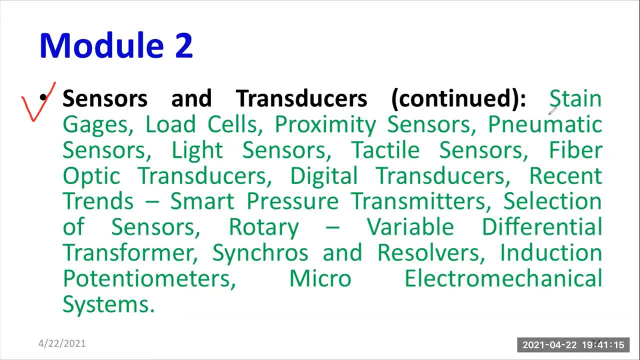 all the things I'll be covering in the second module. So I'm going to explain about strain gauges, then load cells, then proximity sensors, then the transducers. So let us begin. Let me first explain about the strain gauges, which is the mycological data, The strain gauges. 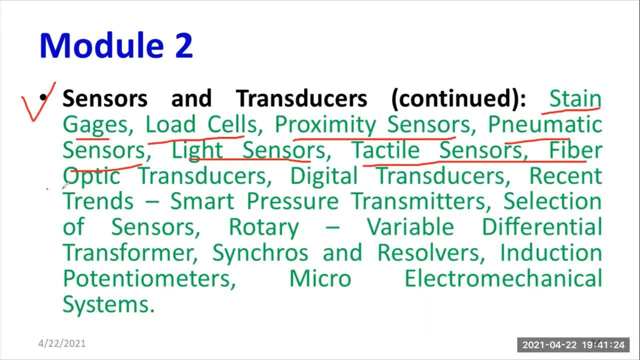 are primarily for the transducers, So live sensors, pneumatic sensors and the light sensors, tactile sensors, fiber optic transducers. It is mainly for ORC communications. Then different type of digital transducers will be familiar and recent trends and smart pressure transmittors. 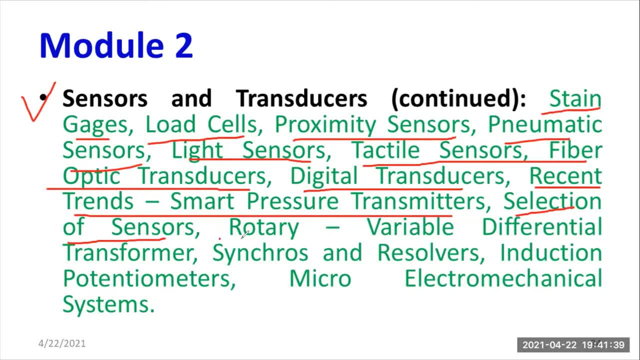 How to select a sensor or a transducer. Then what do you mean by rotary variable differential transformer and applications of rotary variable differential transformer? Then what do you mean by synchro's and the synchro pair characteristics? that is already explained. So the main things. 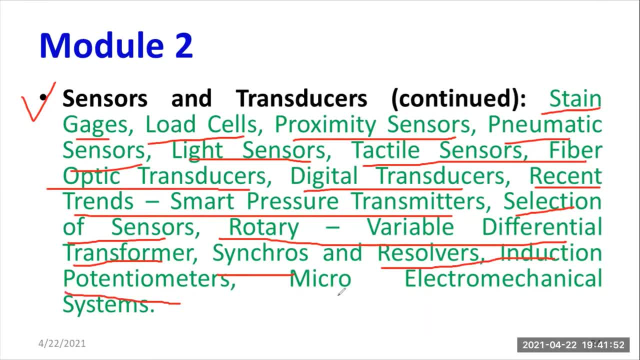 that we are going to consider is Machtoland transducers and the hybridest- democracy transmittable сразу transducers. Okay, So let us begin. We will first look at the popularity, the perception, then induction potentiometers, then MEMS. What do you mean by MEMS? Elaboration of MEMS is 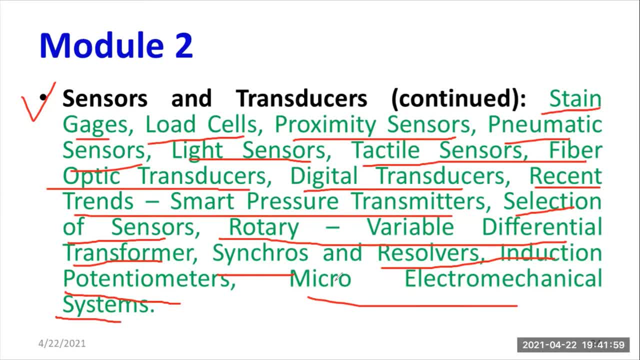 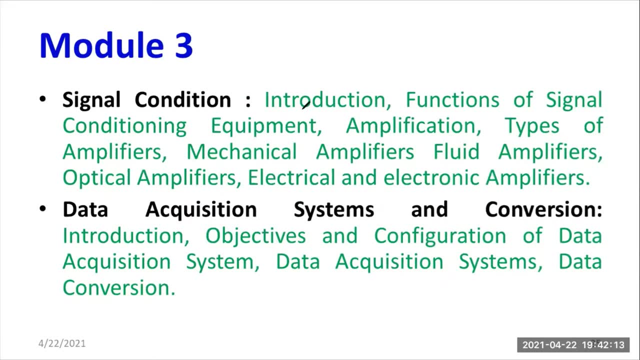 microelectromechanical system. It's a highly advanced topic. I'll be discussing the current trends of MEMS also. So this is the main content which I'll be discussing in second module, And regarding third module, I'll be mainly focusing on the signal conditioning. You know that. 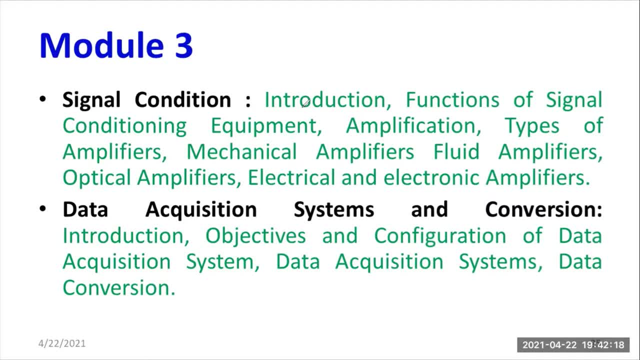 the main component of transducers are: one is sensor, other will be signal conditioning device. So I'll be talking about what do you mean by signal conditioning, Why it is required. So introduction to signal conditioning and the functions of signal conditioning and different type of signal conditioning equipments. What do you mean by amplification? 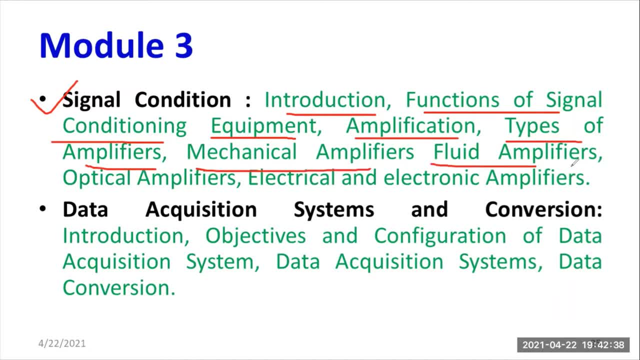 Type of amplifier, such as mechanical amplifiers, fluid amplifiers, optical amplifiers, electrical and electronics amplifiers. So these are all the things which will be belong to the first module of the second module of the second module of the second module of the 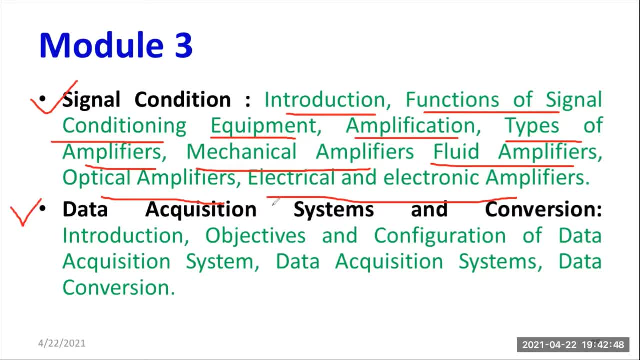 first part of module three. And coming back to the second part, data acquisition system and conversion. Here I'm going to discuss about what do you mean by data acquisition, main objectives and different configurations of data acquisition system. It is one of the cutting edge topic. 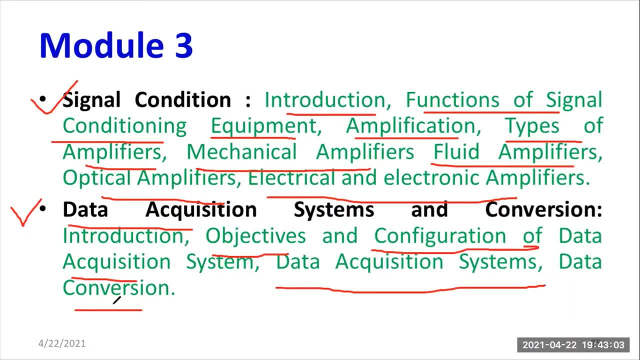 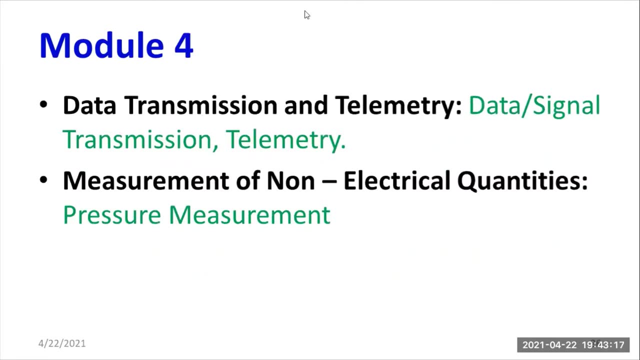 Okay, current trends, then data acquisition systems and data conversions, And I'll be explaining in a simple manner. Anyway, if I talk about transducer, I should have some idea about different type of sensors and the signal conditioning device. Moving on to the fourth module, I'm mainly concentrating on data transmission and telemetry. 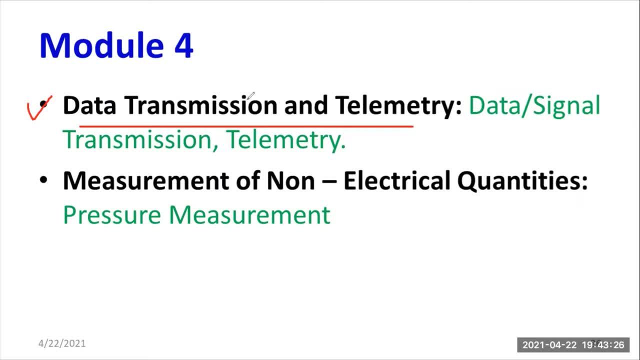 What do you mean by data transmission, How it is correlated to transducers And what is the importance of telemetry And what are the different type of telemetry systems. And from fourth module onwards, I'll be explaining how do you measure non electrical quantities? First, in the foremost, 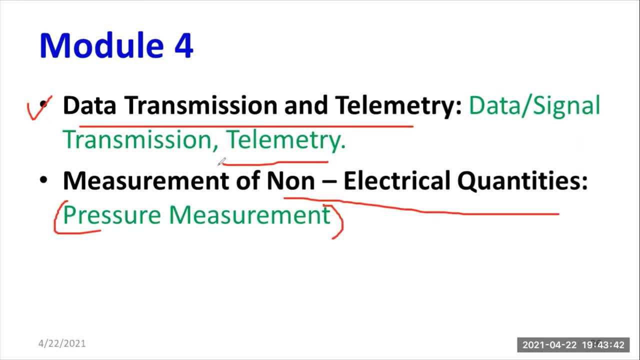 I'm going to explain the pressure measurement. How do you measure pressure? Okay, so in continuation with the fourth module, I'm going to explain the non electrical quantities measurement in the fifth module. also, it is a continuation. Okay, once I complete the pressure measurement directly, I'll 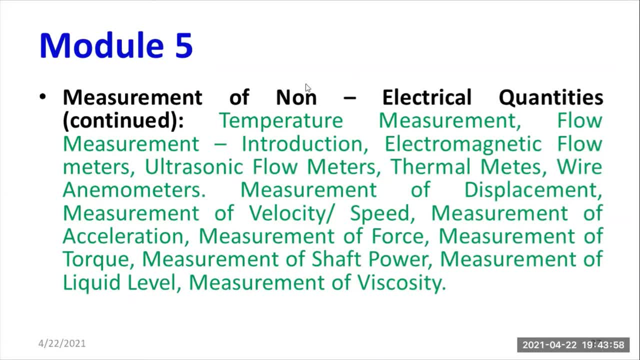 be moving on the different type of measurement of non electrical quantities, such as the temperature measurement, then flow measurement. Okay, I'll be giving a brief introduction- and a different type of flow measurement devices, such as electromagnetic flow meters, then ultrasonic flow meters and the 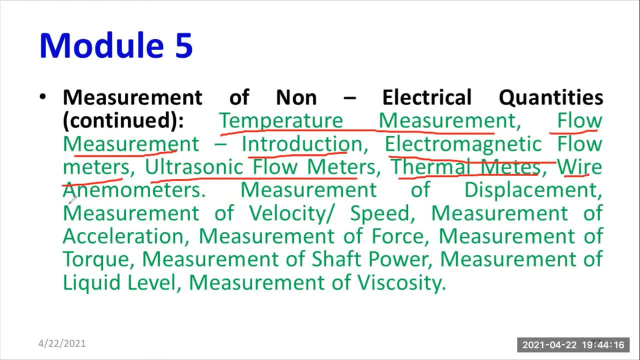 thermal meters, Similarly wire anemometers, etc. And measurement of displacement- that I'm going to explain separately. then measurement of velocity or speed: okay, then measurement of acceleration will be discussed, then, how to measure the force, And how do you measure the torque? And how do you measure? 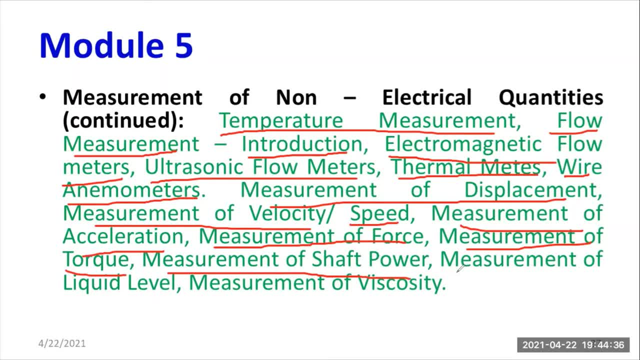 the shaft power, one of the automobile application that I would like to explain. then, measurement of liquid level. how do you measure the liquid level? the measurement of viscosity. So these are the applications in the area of chemical electrical, electrical electrical electrical, electrical. 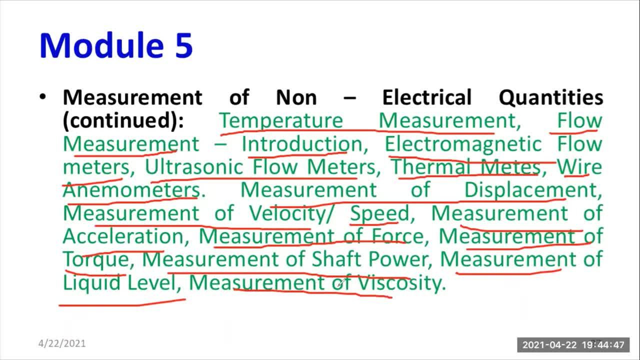 of chemical engineering, especially liquid level measurement, as well as viscosity in the field of chemical engineering. Okay, these are all the things that I'll be discussing in the upcoming days. First, I'll be explaining what is a sensor And what are the types of sensor. Later on, 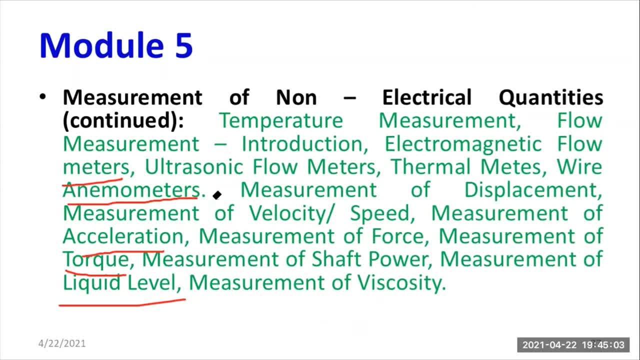 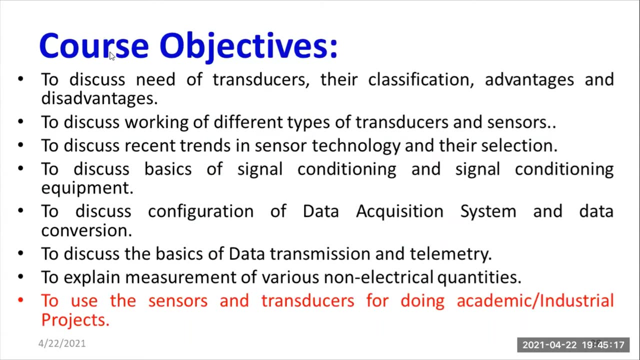 what do? what do you mean by transducer? What is the difference between sensors and transducers? Because many of them are getting confused about the difference between sensors and transducers. that I would like to make clear first. that is our primary objective, So one of the main course objectives are as follows: 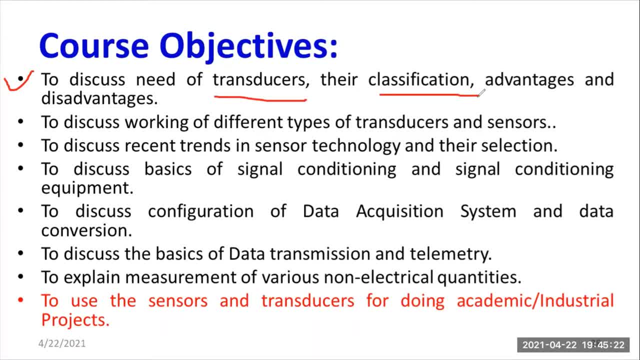 So that is to discuss the need of transducers, their taxonomy pros and cons, And you have to familiar different type of transducers and and it's working. and also you have to familiar the sensors also okay, and you have to bifurcate transducers and sensors and discuss the recent. 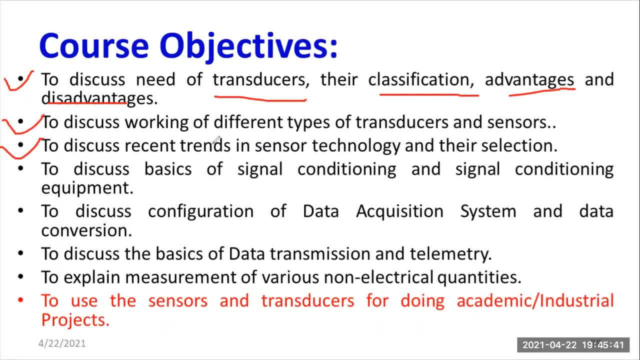 transient sensors, technology and the selection. how do you select the sensors and what are the cutting edge technologies? what are the current trends? that you have to identify And to discuss the basics of signal conditioning device. anyway, in transducer there are two components. The first component is sensor and the second component is signal conditioning device. 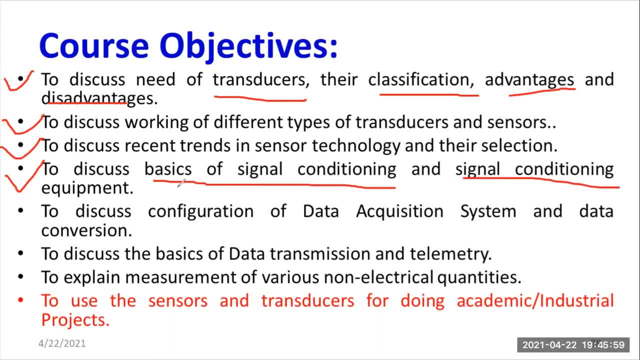 you have to understand the importance of signal conditioning devices. Okay then, to discuss the configuration of data acquisition system and data conversion. that is very important, especially if I talk about antennas: how you are going to transmit the data Antennas? Antenna is one of the examples of transducer. 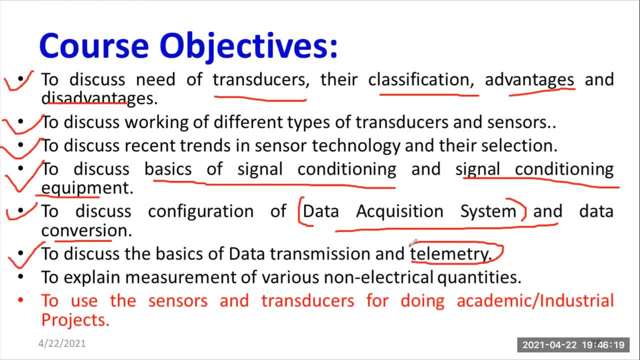 Later on I will be discussing about telemetric system, different type of telemetric system and the basics of data transmission. It will be really helpful for electronics and communication engineering students And to explain the measurement of various non-electrical quantities such as force measurement, torque pressure, displacement, velocity etc. 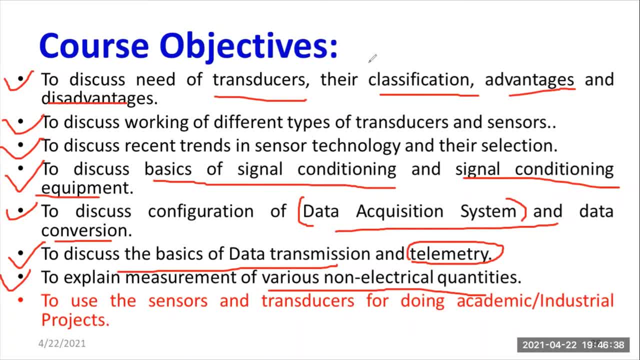 Ultimately, once the course is completed, you can be able to do some kind of useful project for your academics. So that is the ultimate goal. This I am going to imply separately. I am focusing on the last objective because it will be really helpful.